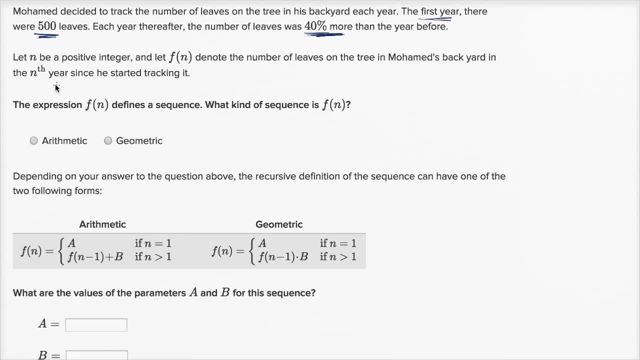 the number of leaves on the tree in Muhammad's backyard in the nth year since he started tracking it. The expression f of n defines a sequence. What kind of sequence is f of n? Some of you might be able to think about this in your head. 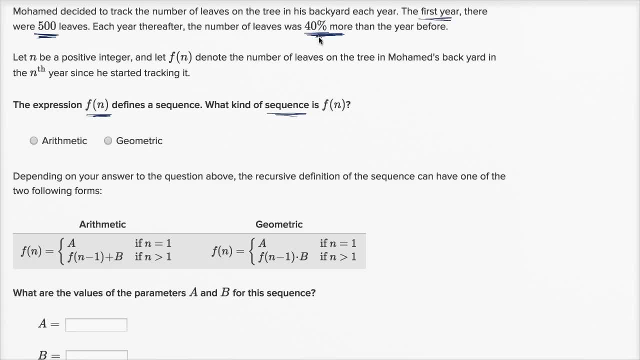 Each successive year, we're growing by 40%. That's the same thing as multiplying by 1.4.. You might say: well, each successive term we're multiplying or dividing by the same number. Well, it's going to be geometric. 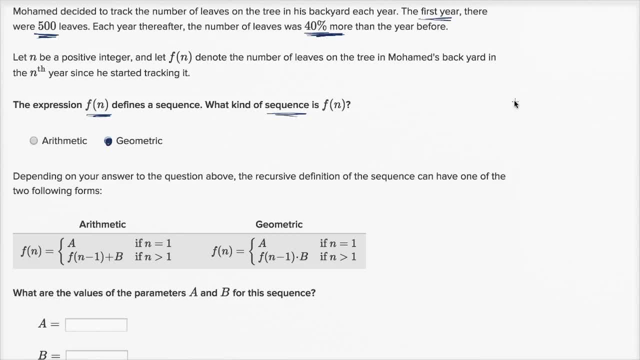 Let's make that a little bit more tangible, just in case. Let's make a little table here, Table. so this is n and this is f of n. An n is equal to one. The first year n equals one. There were 500 leaves. 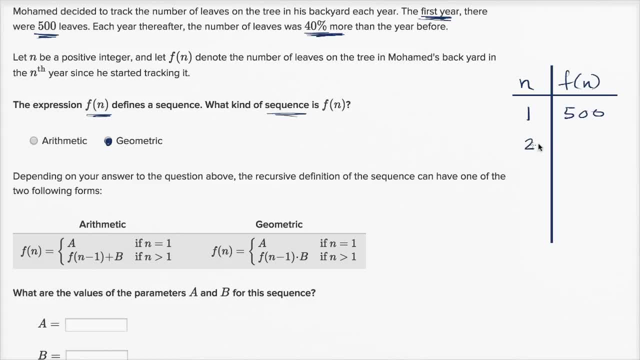 F of n is 500.. Now, when n is equal to two, we're going to grow by 40%, which is the same thing as multiplying by 1.4.. So 500 times 1.4, let's see: 40% of 500 is 200,. 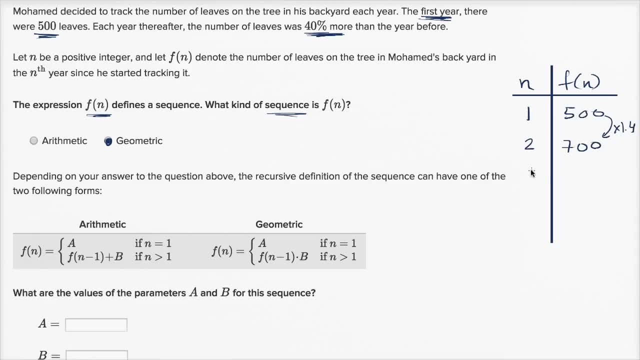 so we're going to grow by 200, so we're going to go to 700.. Then, in year three, we're going to grow by 40% of 700, which is 280, so it's going to grow to 980.. 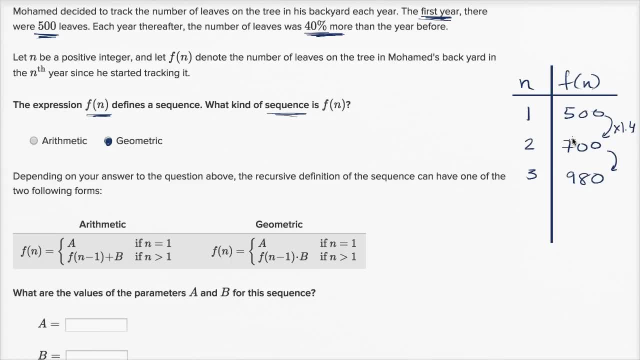 So notice, it's definitely not an arithmetic sequence. An arithmetic sequence, we would be adding or subtracting the same amount every time, but we're not Here. from 500 to 700, we grew by 200, and then from 700 to 980, we grew by 280.. 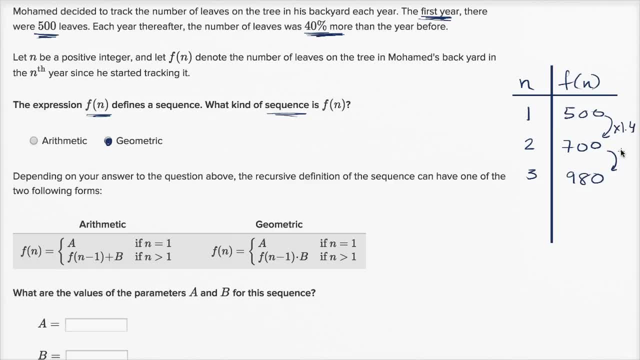 Instead, we're multiplying or dividing by the same amount each time. In this case, we're multiplying by 1.4, by 1.4 each time. so we are clearly geometric, Depending on your answer to the question above, the recursive definition of the sequence. 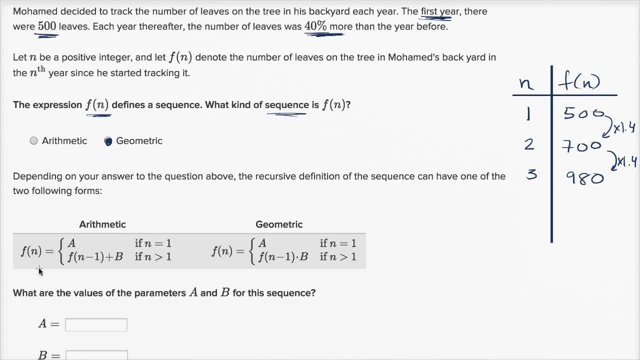 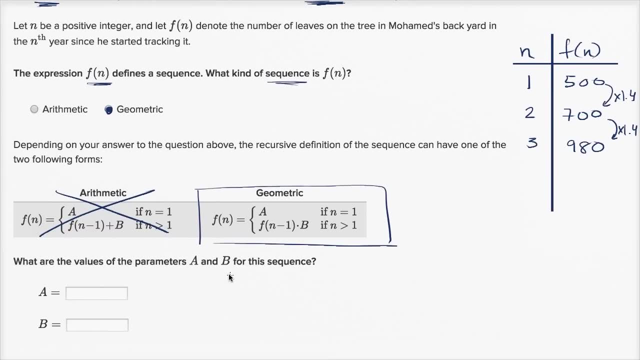 can have one of the following two forms: Well, this is the arithmetic form, which we know isn't the case. so it's going to be in the geometric form. Ask us: what are the values of the parameters a and b for the sequence? 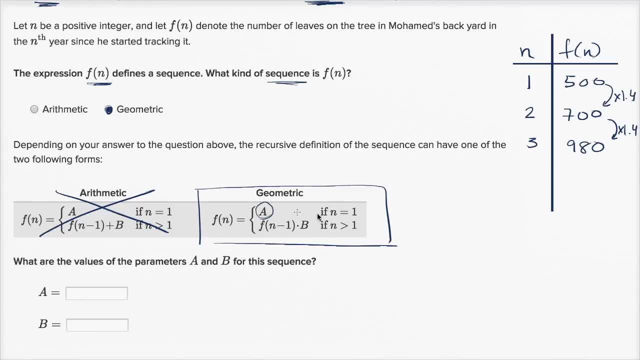 So we have our base case here: F of n is going to be equal to a when n is equal to one. Well, we know that when n equals one, we had 500 leaves on the tree, so a, this a over here, is 500. 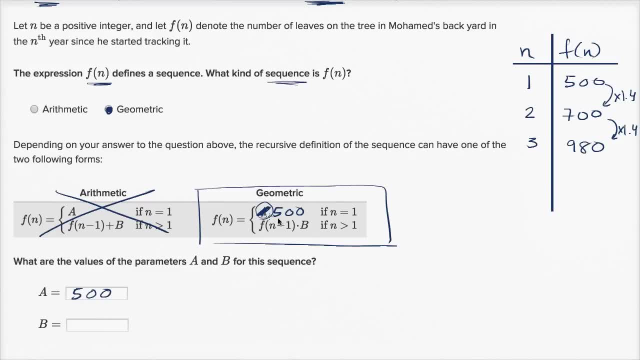 So a is 500. And then, if we're not in the base case for any other year we're going to have, let's see, it's going to be the previous year, The previous year times what Well, it's going to be the previous year. 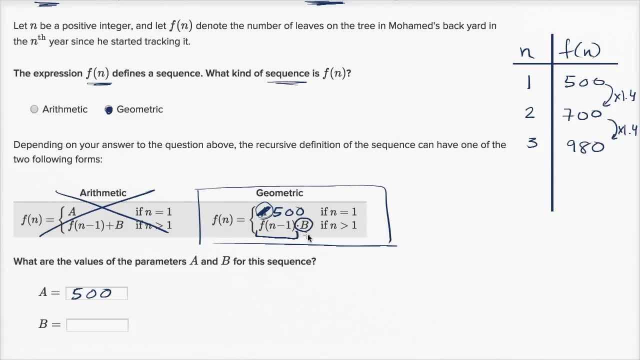 grown by 40%. To grow by 40%, you're going to multiply by 1.4.. So b is going to be 1.4.. You take the previous year and you multiply by 1.4 for any other year. any year other than n equals one. 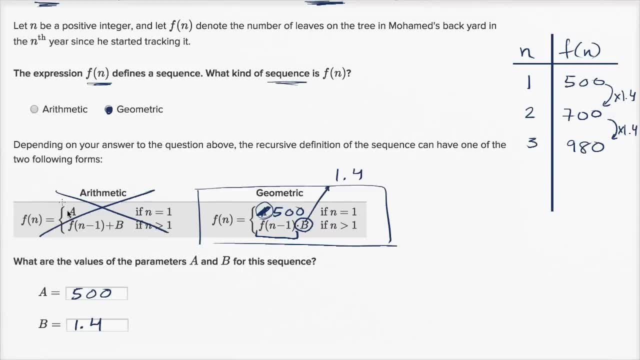 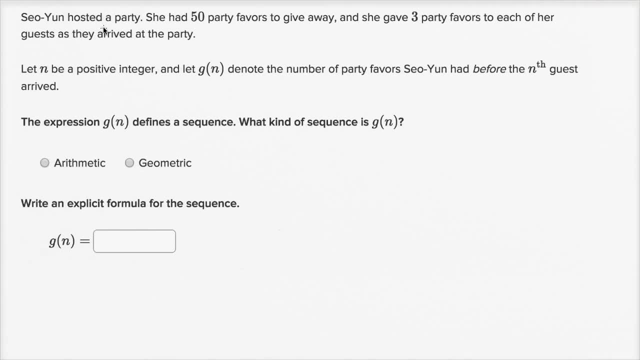 So b is equal to 1.4, and we're done. Let's do another example. This is strangely fun, All right. So this says Siu Yun hosted a party, She had 50 party favors to give away and she gave away three party favors. 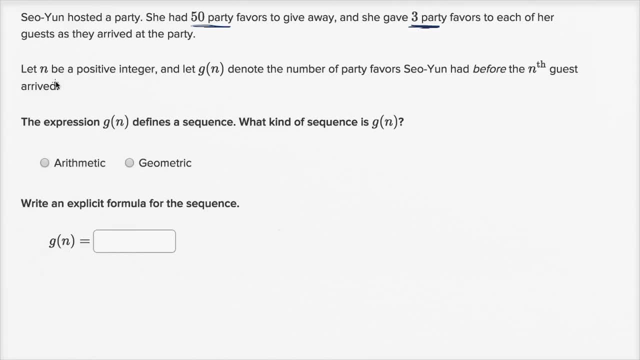 to each of her guests as they arrived at the party. Let n be a positive integer and let g of n denote the number of party favors Siu Yun had before the nth guest arrived. All right, actually, before I even look at these questions, 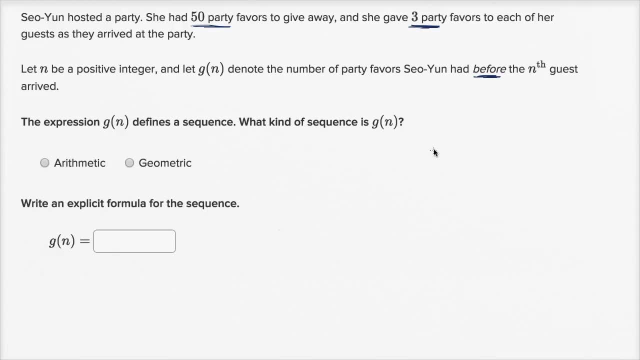 let me make a table here, because they're saying: before the nth guest. I want to make sure I'm understanding this properly. So this is n and then this is going to be g of n, g of n, right over here. 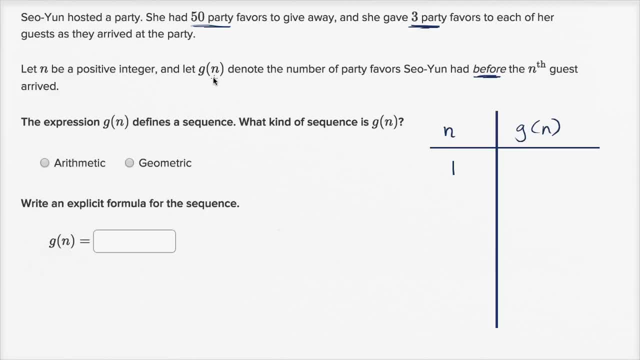 So, when n is equal to one, when n is equal to one, g of n is going to be, or g of one is going to be, the number of party favors Siu Yun had before the first guest. Well, before the first guest, she had 50 party favors. 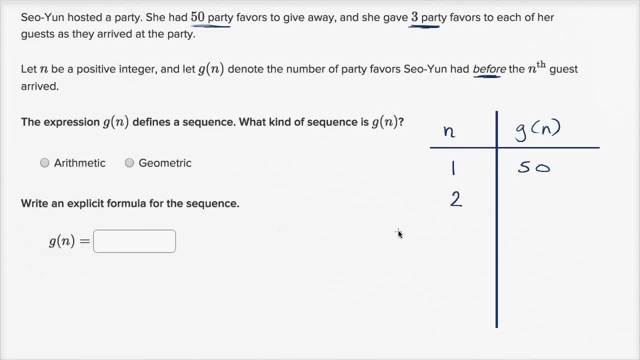 She had 50 party favors. Now the second guest comes. Now the number of party favors she had before the second guest. well, she had to give three to the first guest, so she's now going to have 47 party favors. Now, when n is equal to three, 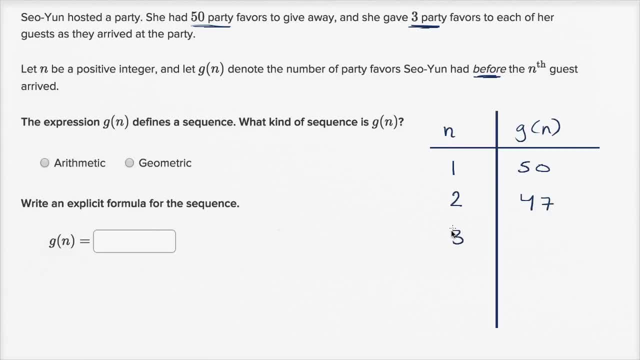 how many party favors did she have before the third guest? Well, she would have had to give party favors to the first and second guests, who each got three, So she would have 44. And I think you see the pattern. For every time n, when n equals one, g of n is 50,. 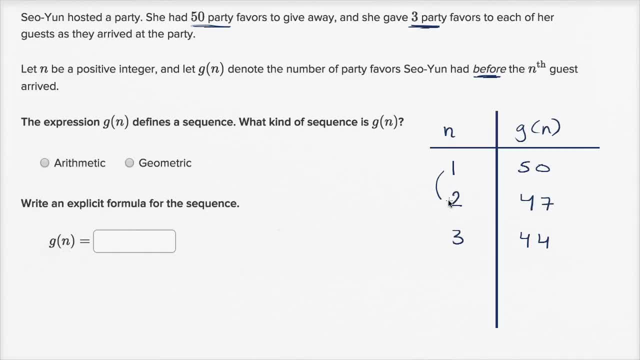 and every time we increase n by one, every time we increment n, we are increasing g of n by plus three, by minus three. I should say She's giving away party favors Minus three, minus three. So because the difference between successive terms